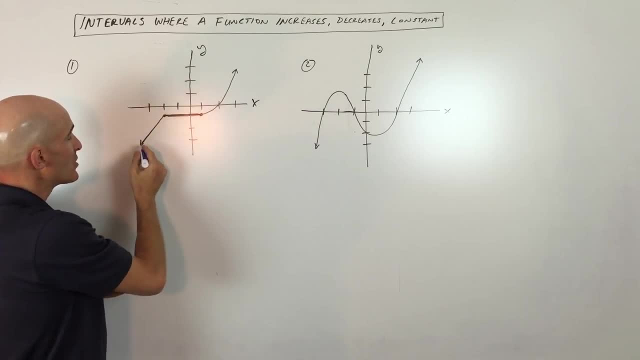 about going from left to right or from low to high, And so here you can see this is going off towards negative infinity. So we have negative infinity, okay, all the way up to where x is negative 2, okay. Now, when you do the increasing and decreasing intervals, you want to make them. 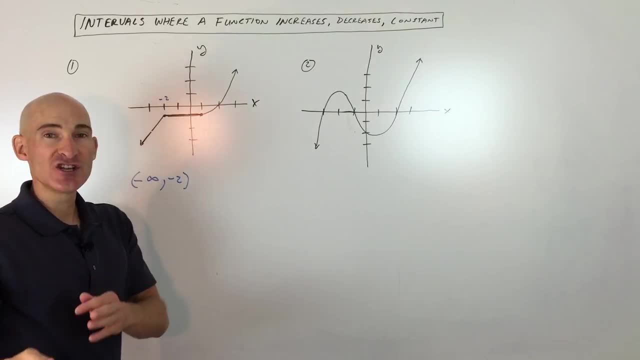 open intervals. You don't want to include the endpoints. That's where it's changing direction. It's changing from increasing to decreasing or increasing to constant. So you always want these to be parentheses, Not the square bracket where it includes that point. Okay, so then also we can see that the 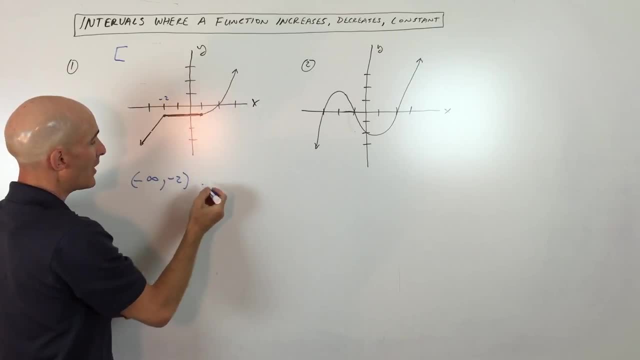 graph is going up to the right here: when x is greater than 1, okay, So we're going to put union 1 to positive infinity. Now where students sometimes go off the tracks is they'll start thinking about the y values. So they might say: well, it's increasing up until y equals negative. 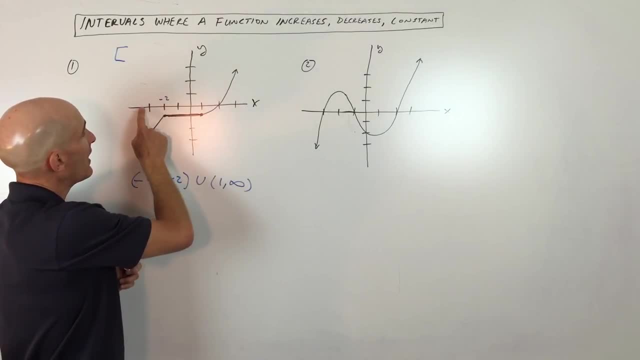 1. That's not correct. You want to think about, you know, what the x values are okay and what the y values tell you. So you want to think about what the x values are okay and what the y values. 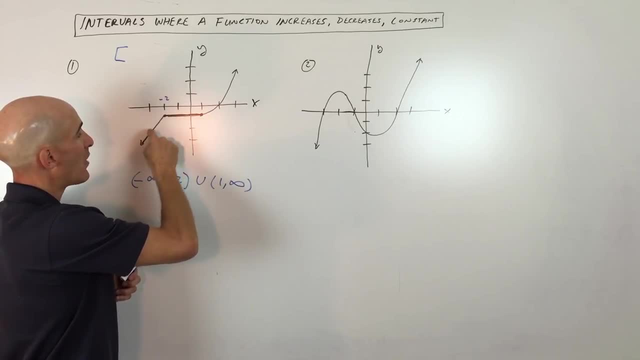 tell you. So you want to think about what the y values tell you. So you want to think about what the y values tell you. So you want to think about what the x values tell you. See, the y values are increasing. See, as this graph is going up. see, the y values are increasing only when x is from. 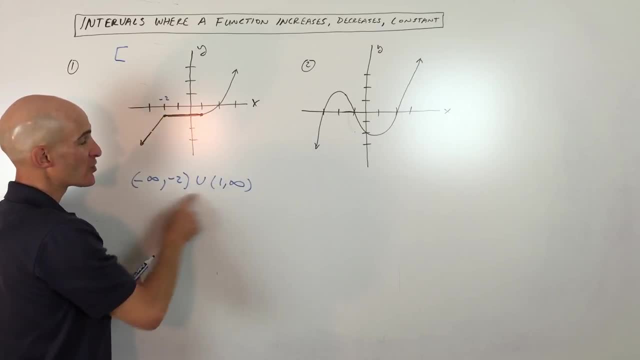 negative. infinity to x is negative, 2.. So these really represent the x values where the y values are increasing or the graph is going up. Okay, so this is the increasing. Now you can see here it's constant: from x is negative 2 to x is positive, 1.. So we're going to say constant. I'll 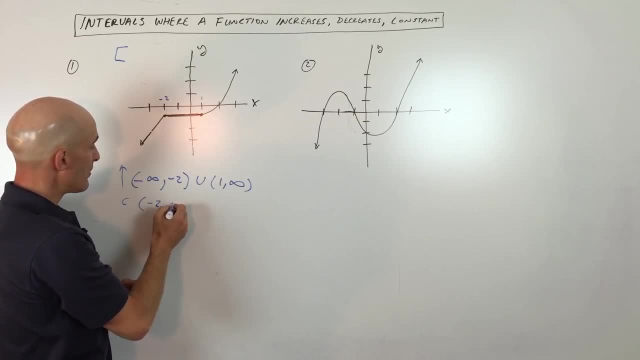 just put a c there and we're going to go from negative 2 to positive 1.. Again, notice we're using the parentheses, the open interval. It doesn't include the x values, So we're going to include the endpoints. whenever you do these increasing, decreasing and constant intervals. 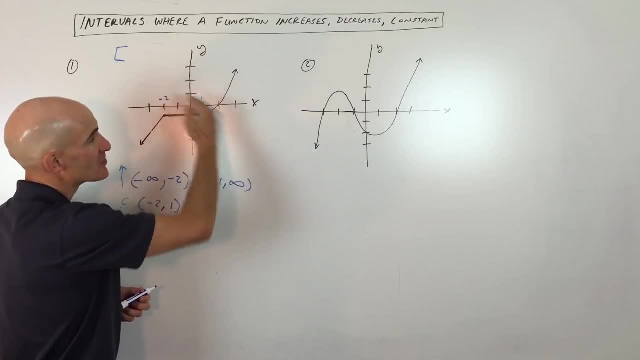 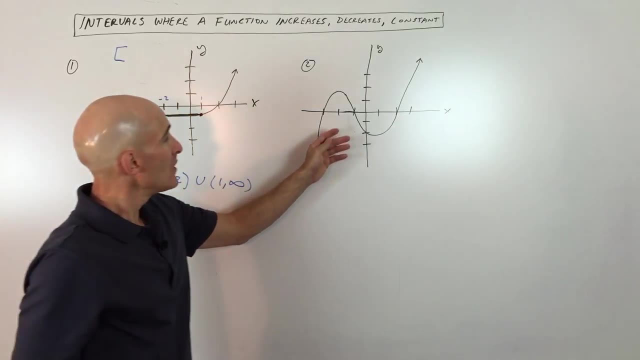 And then where is the graph decreasing? Well, you can see nowhere is it going down to the right? So it's just going to have these increasing and constant intervals. Okay, let's look at example number two. Now, this one, we're looking at where it's increasing. So you can see it's going up.